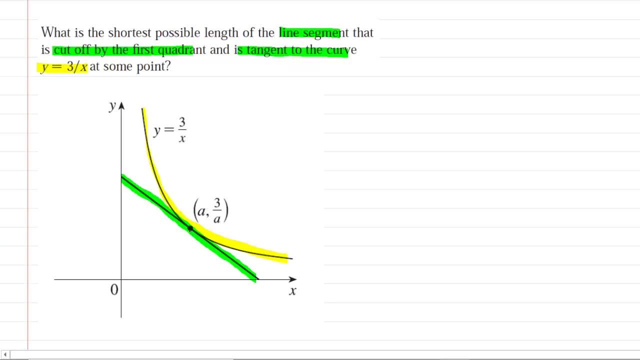 of an arbitrary selection of variables. So basically, the x coordinate of that point we are calling a, And then the y coordinate we obtained by plugging a into this equation. We can see that at that point the green line segment and the yellow curve intersect. at that point, because the 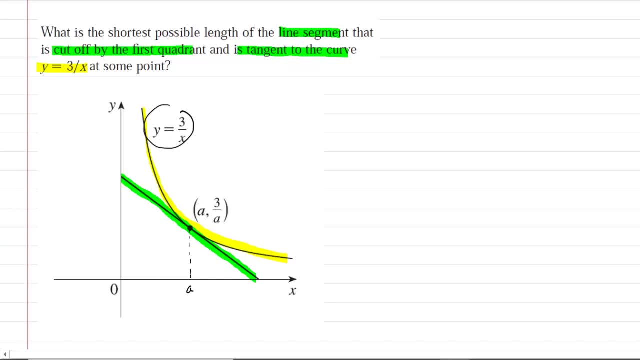 green segment is tangent to the yellow curve, Because they intersect, then they have the same y coordinate And therefore, to find that y coordinate, we can plug a into the equation. So that's where we're getting the 3 over a from. So basically, right, there would be 3 over a. 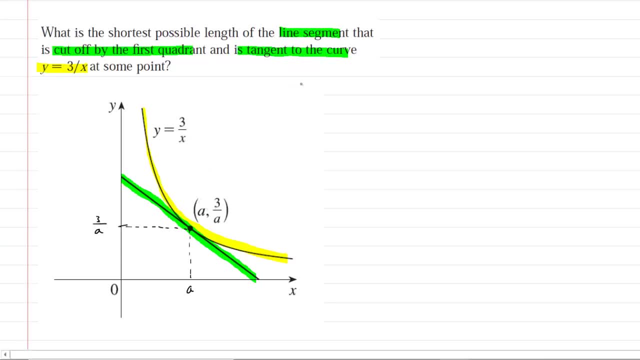 So this is the picture. That's the picture that we have drawn, Step 1.. Step 2 is to come up with a couple of equations, And one equation that we're going to need to come up with is what I like to call the constraint equation. 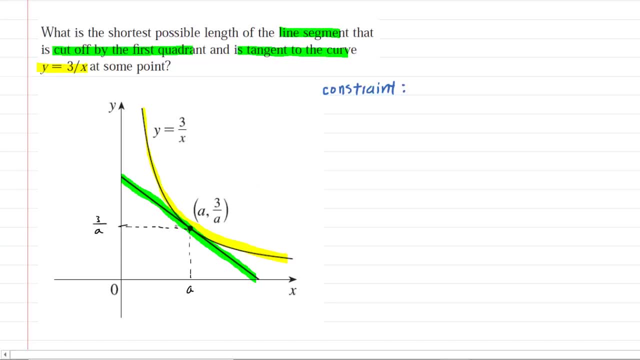 Now, in this particular case, the constraint equation is actually going to be the equation of that green line segment. So we're going to have to find a way to develop an equation of the green line segment. We know from a pre-calculus course that the equation of a line is going to be the equation of the green line segment. 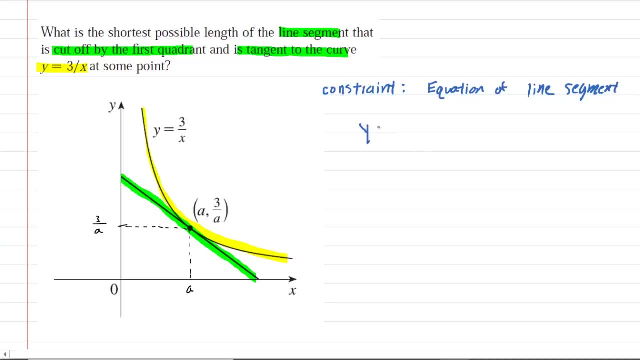 So we're going to have the equation of a line is written in a sort of point slope form. So it would be: y minus y1 is equal to the slope of the line times x minus x1.. Let us also recall that x1 and y1 would be a point on the line. So we're going to write that down on the side here: x1 and y1 are a point on the line segment. 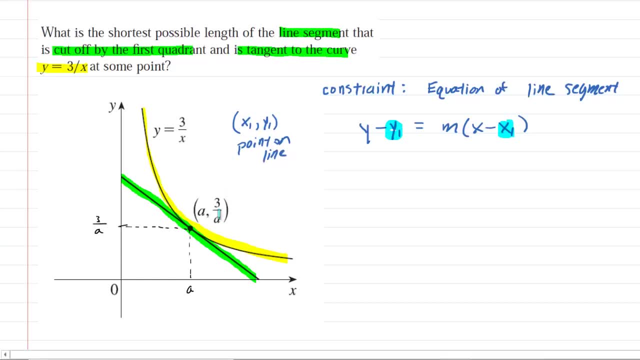 Now we've already discussed that. we have a point on that line segment right here. So this a is going to be our x one, essentially, and then the three over a is going to be our y one. So why don't we go ahead and just plug those? 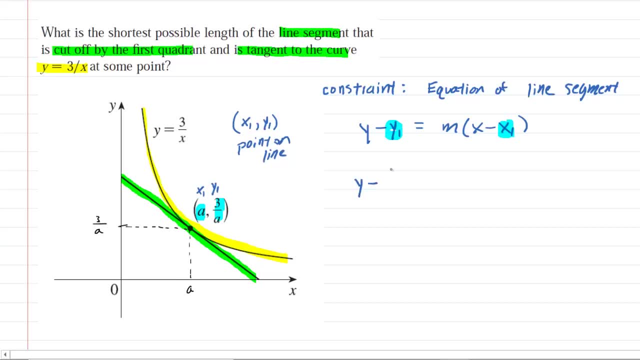 into the equation of our line segment. So again, the y one is three over a. This will equal the slope of the green line segment times x minus a. That was the x coordinate of a point on the green line. So we're doing pretty well so far. 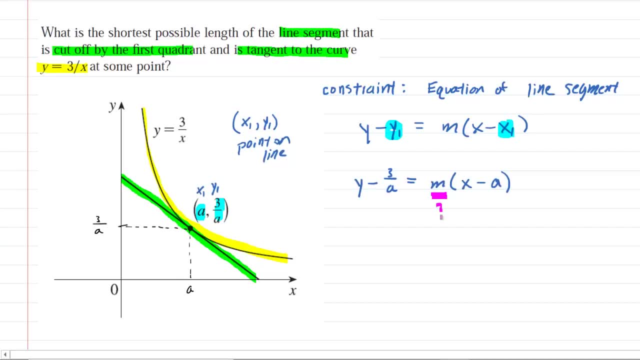 but what we really need next is the slope of this green line segment That becomes our next challenge is to try to fill in something for that slope. Now, a key idea here- from the picture, hopefully, we can see- is that the slope of the line segment is going to equal. 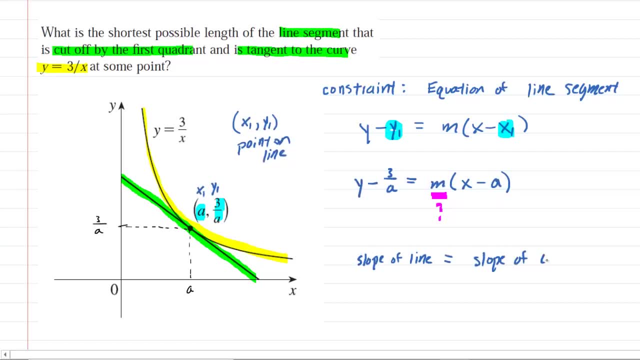 the slope of the curve at that particular point right there. That's kind of the definition of a tangent line is that the slope of that tangent line is equal to the slope of that tangent line, to the slope of the curve that it intersects. So to get the slope of the line, 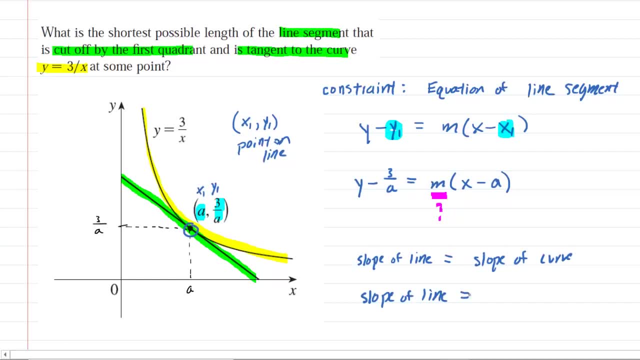 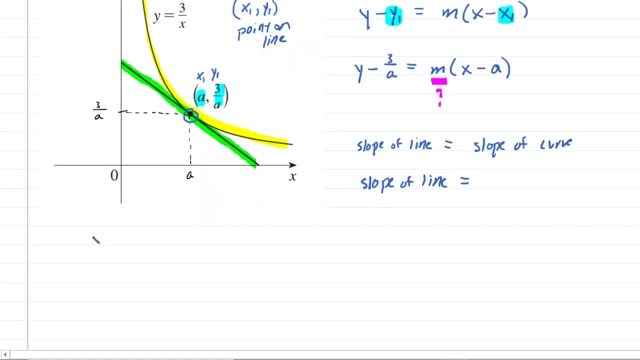 we're gonna actually find the slope of the curve. So that's what we're gonna do next is find the slope of the curve. Let's come down here and talk about how to find the slope of the curve. Now we know the curve has the equation y equals three over x. 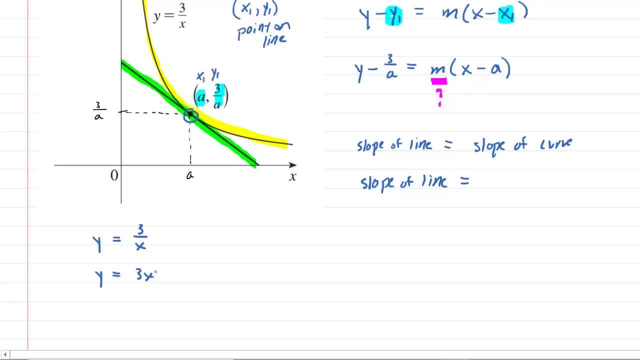 We can certainly rewrite that as y equals three x to the minus one, And then, since we're looking for the slope of the curve, we need the derivative, And that is what calc one is all about, is finding derivatives. This is a simple one, isn't it? 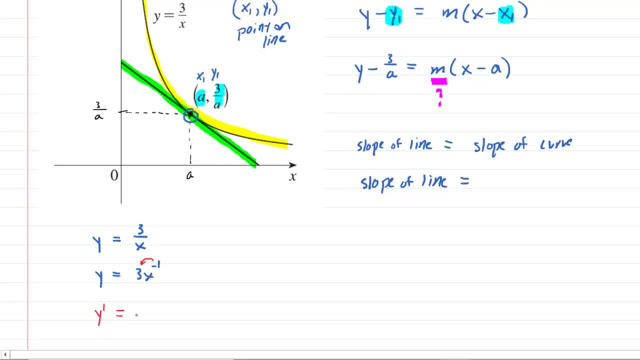 Because it's just a power rule. So you're gonna multiply negative one by three to get negative three, x, and then subtract one from the previous power to get negative two, So we can actually rewrite that as negative three over x squared. Now recall, at this particular point: 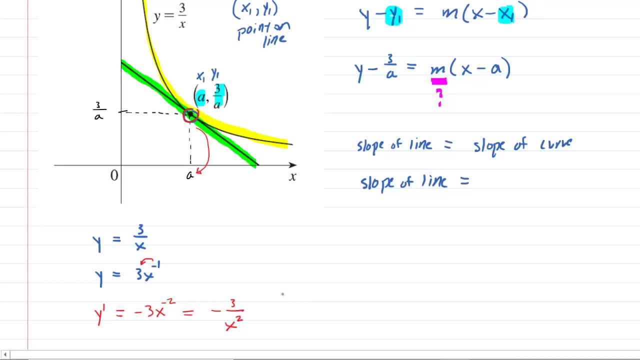 the x coordinate of that point is actually symbolized by a, So we can go just a bit further here and say that the slope at the point a would equal negative three over a squared. That's the slope that we're gonna be substituting in. 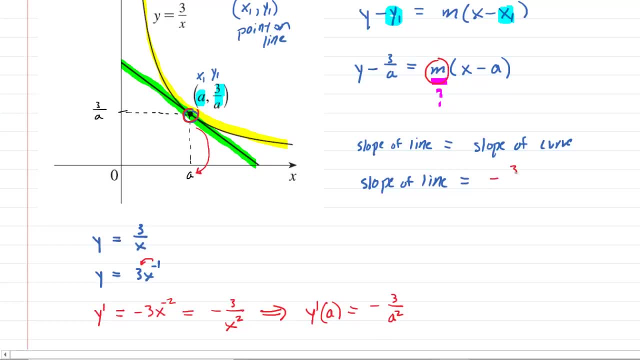 right there, because the slope of the line is equal to the slope of the curve. at that point negative three over a squared. So we can swing down here and write the equation a little bit more here: Y minus three over a is equal to our slope of the green line. 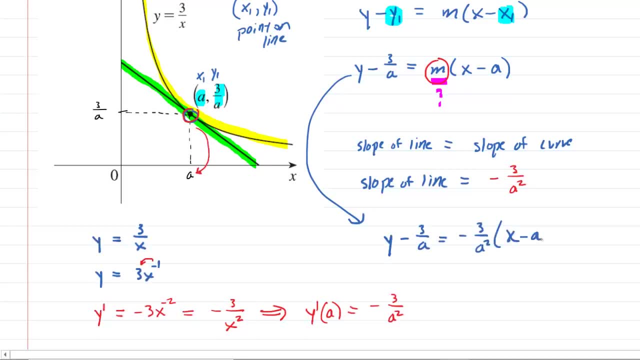 basically being a whole segment, times x minus a. So that's pretty good. We've got the equation of the line in terms of a. What we're going to do next is try to think about the distance or, I suppose, the length of that line segment. 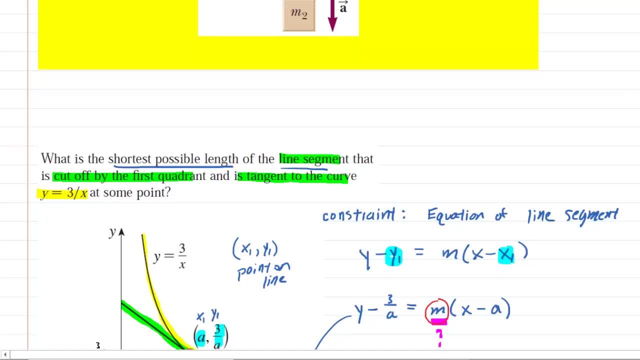 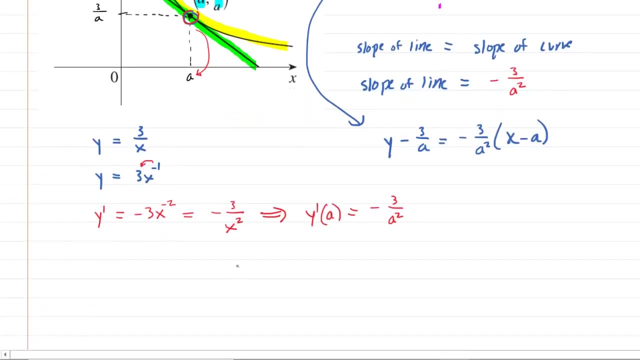 After all, if you go back up to the question, we need to find the minimum length of that line segment. So we need a new equation segment And this becomes what I like to call the objective equation. Our objective is to minimize the length of that line segment. Now we probably have learned that the length or distance of a line 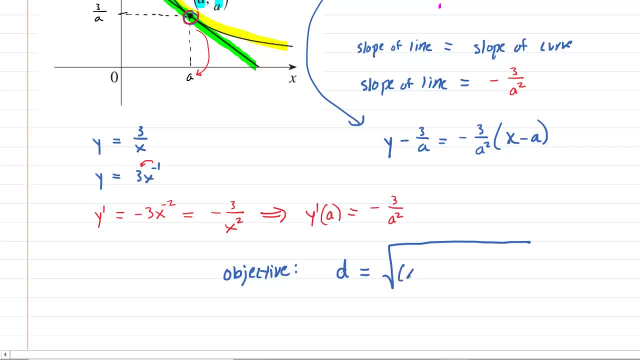 segment is equal to the following equation: This can be developed by using a Pythagorean theorem. We will skip that development and just assume that we have learned this distance formula, And so what we're going to do is plug into that distance formula. But to do so, 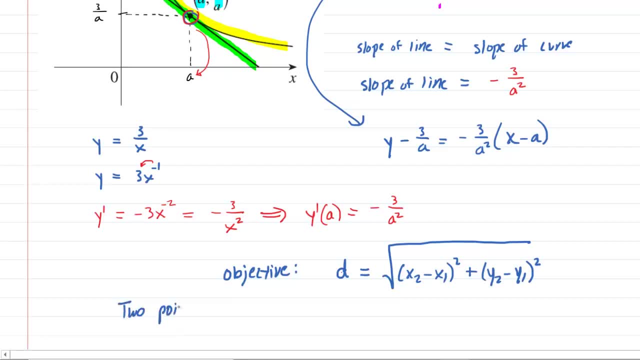 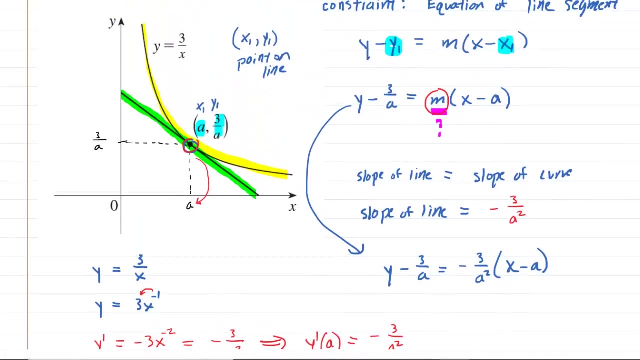 we need to find two points on the line. Now, if we go back to our line, we can perhaps mark a point right here. This is the so-called y-intercept, And then we would have another point down here. This could be our x-intercept. Notice, we're using these two points because we need the. 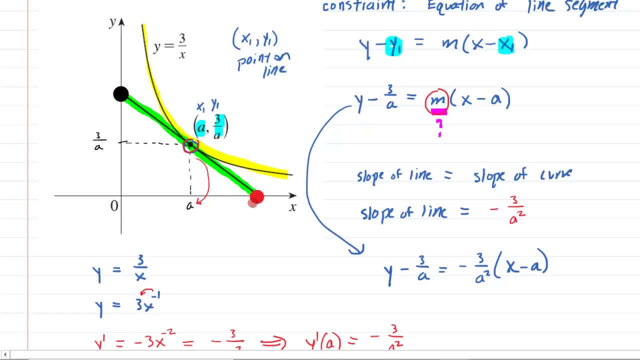 entire distance formula And so we're going to plug into that distance formula And so we need to find the entire length from that y-intercept to that x-intercept. That would represent the length of that entire line segment. So we need to find those. We need to find those. 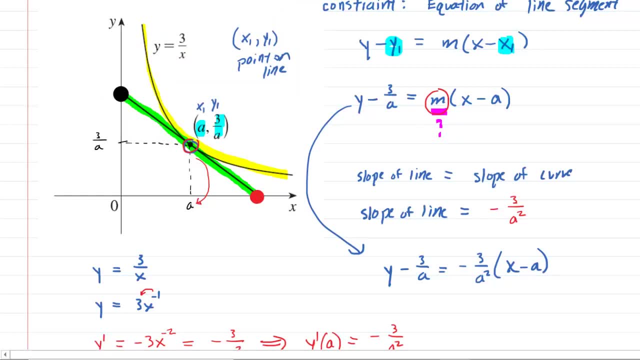 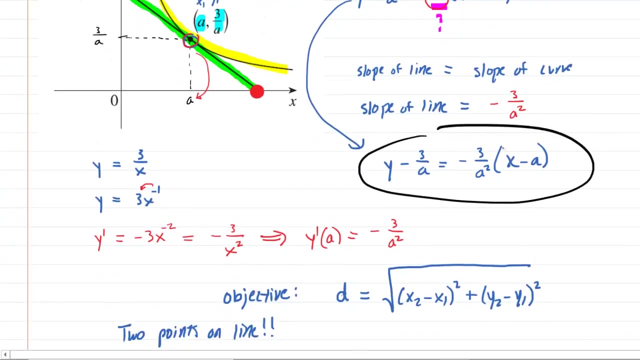 or at least expressions for the y-intercept and for the x-intercept. Let's find the y-intercept. Recall: at the y-intercept, the x-coordinate is equal to zero. That is always true for a y-intercept. So let's go to our equation, this equation for the line, And we're going to find the y-intercept. 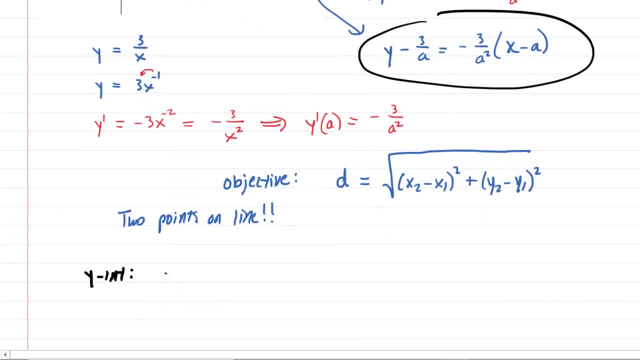 by plugging zero into that equation for the x. So we'll have: y minus three over a equals negative three over a squared times. zero minus a. Now, of course, zero minus a is just negative a, So we're going to have: y minus three over a is equal to negative three over a squared times. 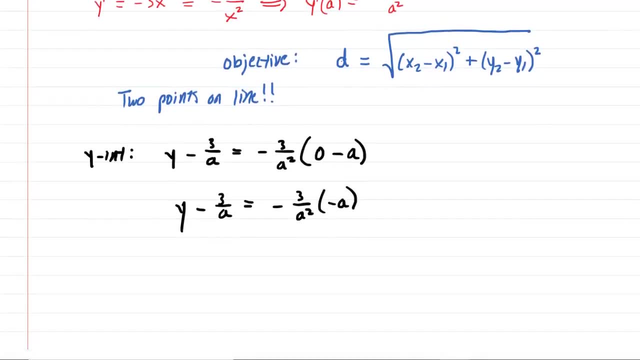 negative a. We can clean this up a bit, can't we? Because you've got a negative multiplied by a negative, so that's going to make it positive. Also, you can cancel a factor of a here and one of the factors of a in the denominator there. So on the right-hand side. 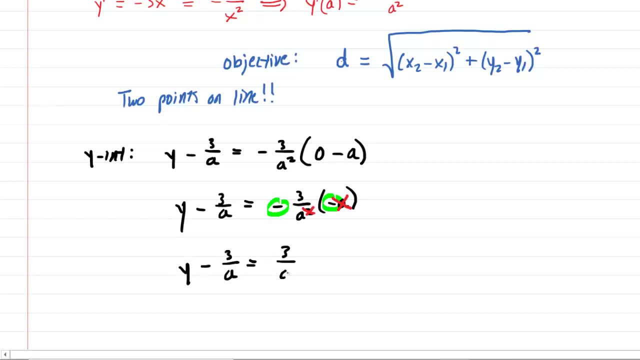 you will have positive three over a, And then, if you add three over a to both sides, you're going to have three over a plus three over a, which is six over a. So, in conclusion, the y-intercept is located at: 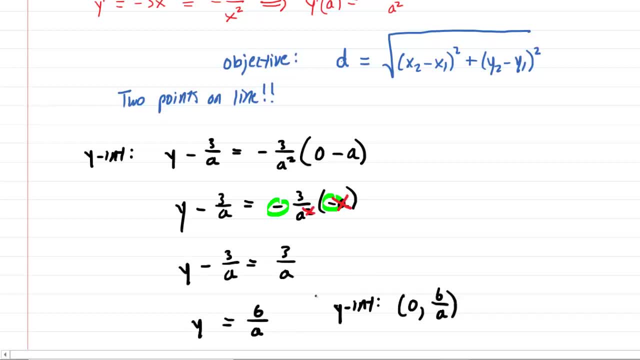 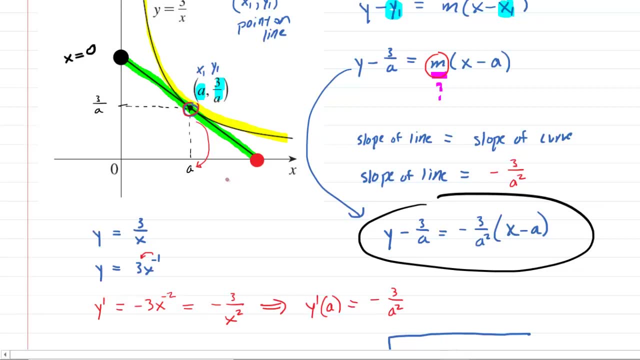 zero comma six over a. So that's a good thing to know. We also need the x-intercept. We go back up to our picture. Here's the x-intercept. We know that to find an x-intercept you're going to let the y equal zero. So let's do this all over again, but this time. 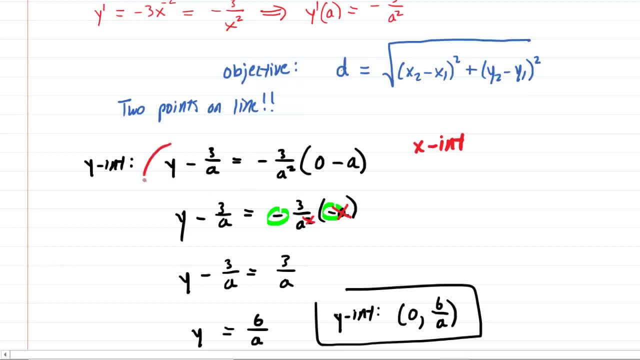 we're going to let the y equal zero. Remember you're plugging into the equation of the line right here. So letting the y equal zero, we would have. zero minus three over a is equal to the right-hand side, which is negative. three over a squared times x minus a. 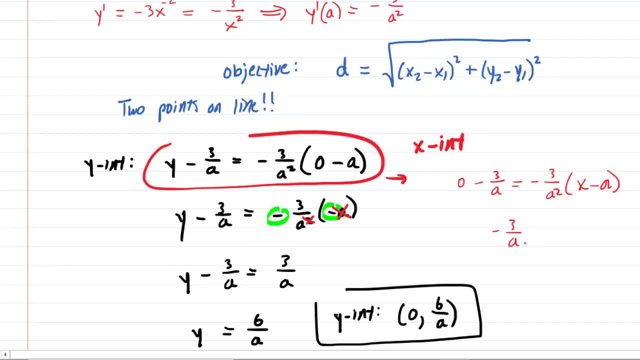 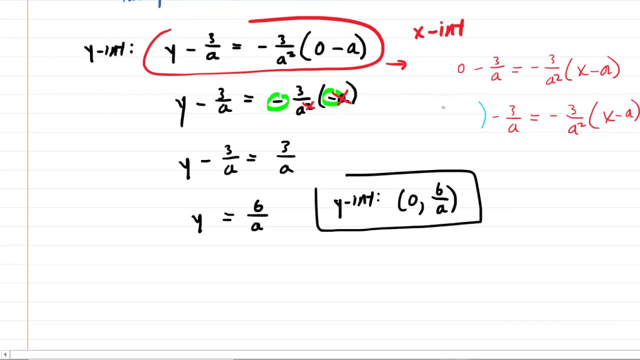 The left side simplifies to: negative three over a equals negative three over a squared x minus a. This is a little more annoying, I think, to try to solve this for x, but maybe what we can do to both sides here is multiply by. let's see, we want to cancel. 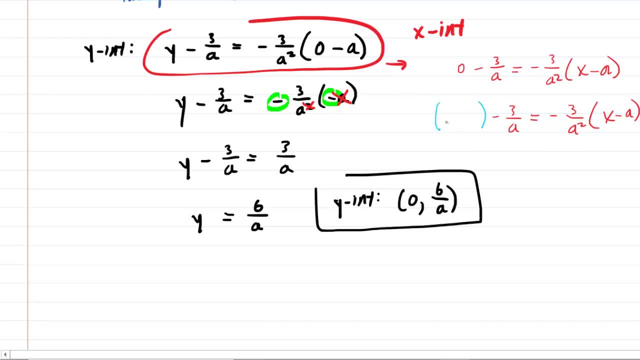 out this negative three over a squared. So we'd have to multiply by. let's see, we'd have to multiply by the reciprocal. Why don't we multiply both sides by negative a squared over 3.. So we're going to try to squeak that in here. You're going to multiply this side by the reciprocal. It's going. 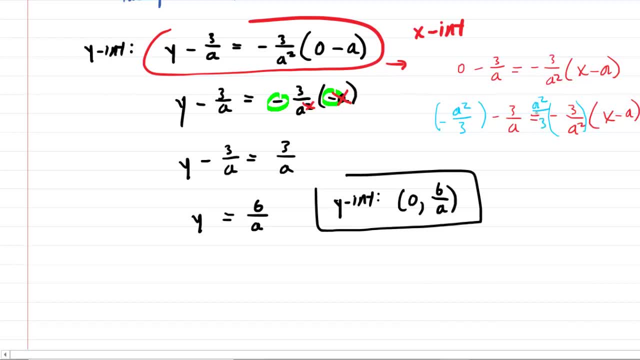 to be a squared over 3, but it's negative. Sorry that's a little messy, but the idea is that this 3 will cancel that 3, and that negative a squared will cancel this negative a squared. So the right hand side, if we continue down here below the right hand side, just becomes x minus a. So I 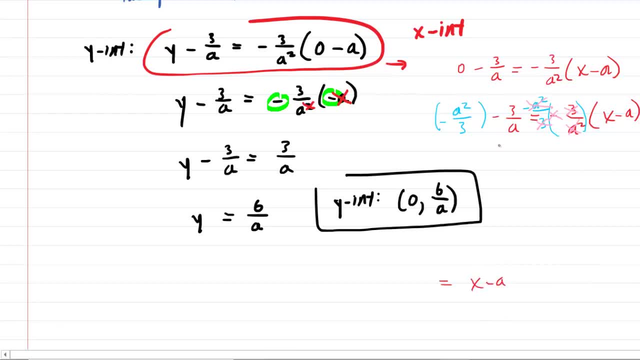 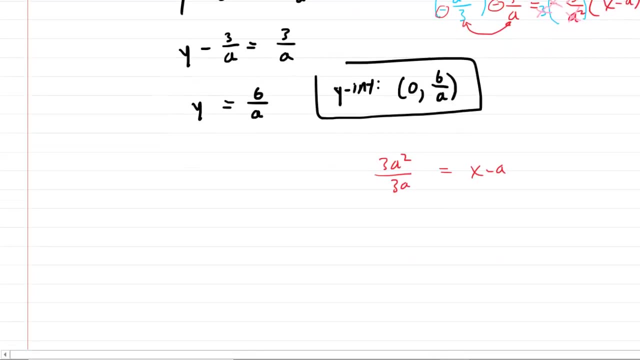 suppose we don't even need the parentheses. The left side. let's see here: you're going to have a negative times a negative. That will become positive. You'll have 3 times a squared, So that's 3 a squared over. And then down here, 3 times a is just 3 a. Let's reduce the left side further: The 3s. 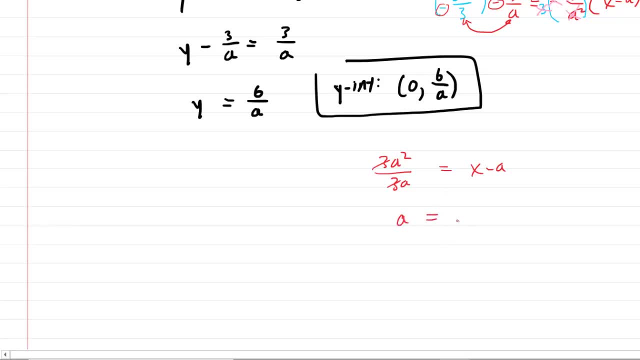 cancel. A squared divided by a is just a. So we have this little equation and then we can add a squared over 3 a squared. So we're going to have a squared over 3 a squared. So we're going to add a squared over 3 a squared. So we're going to have a squared over 3 a squared. So we're going to 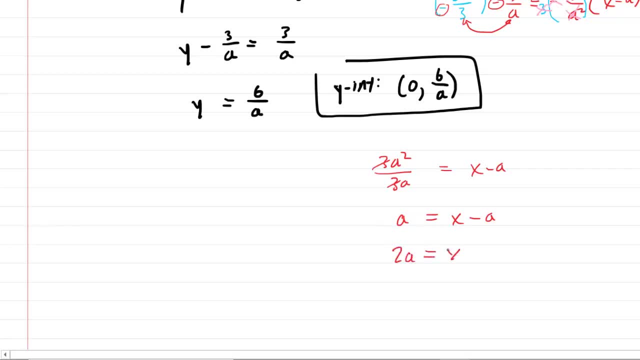 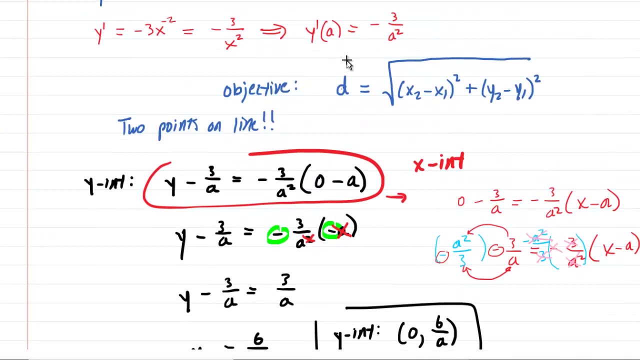 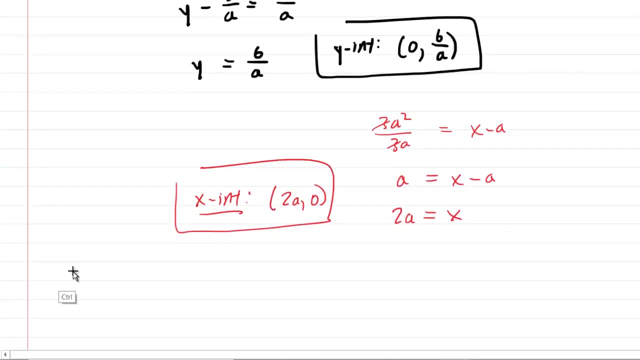 to both sides and we can see that the x intercept is actually located at 2a. so, in conclusion, the x intercept is located at 2a comma 0.. now we can go and use our objective equation. remember it was our objective to minimize the distance between those two points, between the y intercept and the 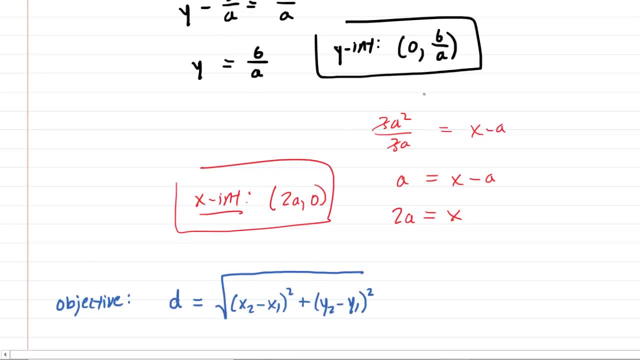 x-intercept. so we're going to plug in. we can perhaps call the x 2 y 2 this point here, the x-intercept and then the y-intercept can serve as our x 1 y 1. it would work either way, so here: 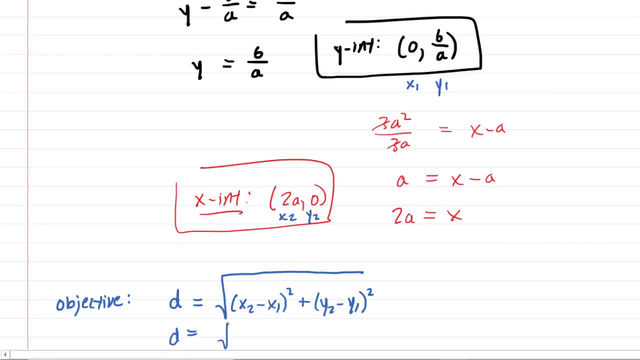 we go, we're going to plug into the distance formula and it's going to get a little messy here. but x 2 is 2a minus x 1, which is 0, and then we square it: y 2 is 0 minus y 1, which is 6 over a, and then that's squared. okay, this is getting us somewhere. we. 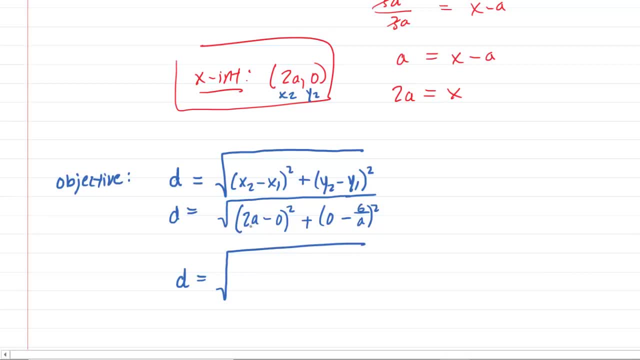 have the objective going on here. we can simplify it: 2a minus 0 is 2a, but then you square that. you get 4a squared plus. you're going to end up squaring a negative 6 over a. you can do that on the side, if that helps. squaring the negative 6 gives us positive 36. squaring a gives us a. 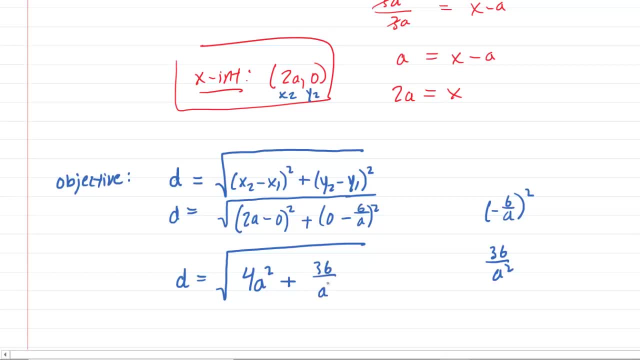 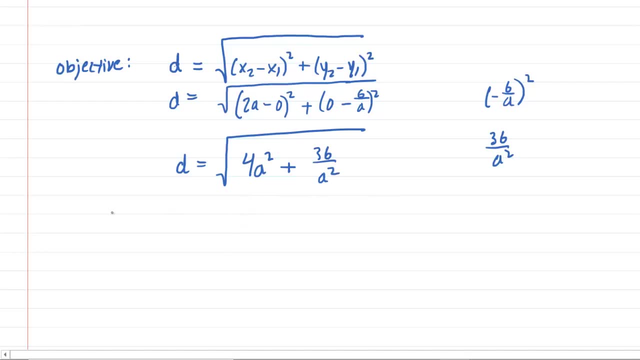 squared, so this becomes a 36 over a squared. good, now, this is our objective is to find the value of a that would minimize this distance. that's what we're trying to do: is find that value of a that would minimize this distance. but it turns out that this would get a little messy because we have the square root. 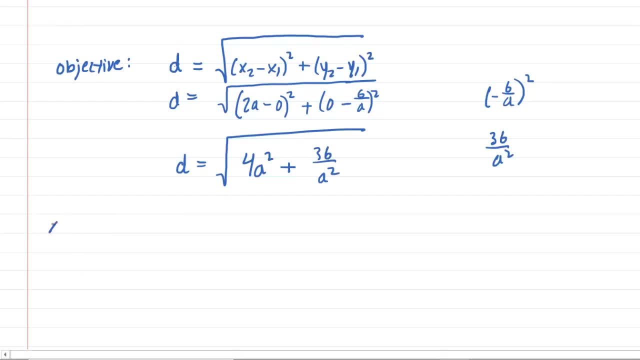 so there's another little idea that we can do or that we can utilize here, is that, rather than minimizing d, we can actually minimize d squared, and so long as we minimize d squared, that in turn will also minimize d, and so it makes the math just a little bit easier. rather than trying to minimize d, 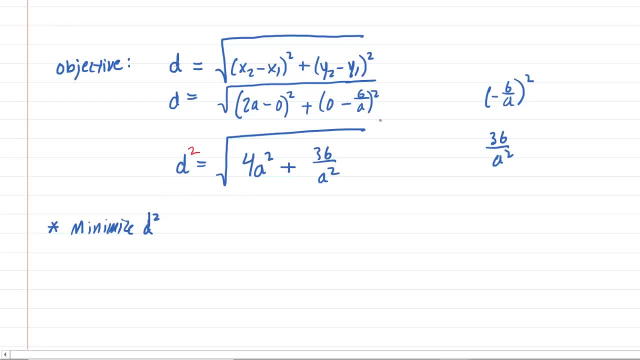 we're going to minimize d squared, so what we'll do is square both sides of this equation. we can see then that d squared becomes simply 4a squared plus 36 over a squared. instead of 36 over a squared, you'll find it useful to actually write that as 36 a to the negative 2.. very good, so this is the new objective of this equation. 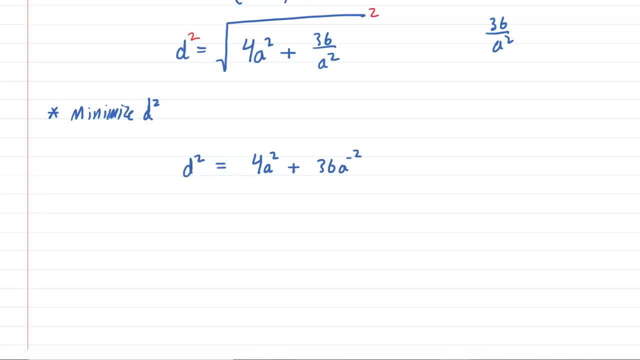 new objective. We've rewritten it in terms of d squared. Now we need to find the value of a that minimizes this function basically, And so this is where we have to use some methods from earlier in the chapter: finding a minimum point. And so you recall that to do that, you have to differentiate. 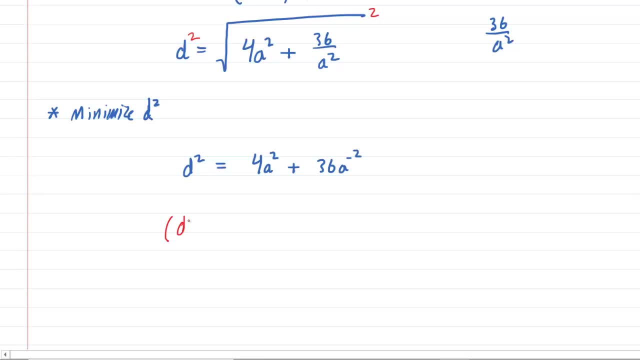 You have to do the derivative of both sides. So the left side you could basically just write as d squared prime. That's just representing the derivative of our quantity d squared. The other side, you're going to do some power rules, So the derivative here becomes 8a, And then over here. 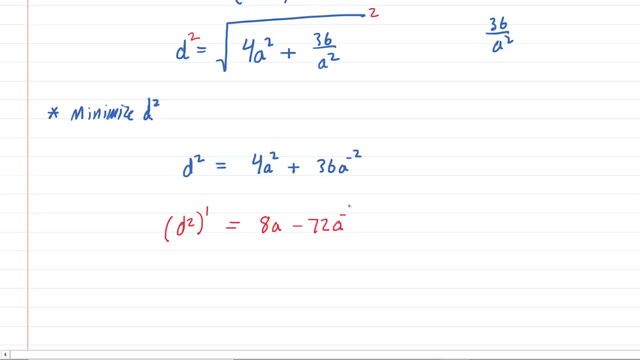 this becomes minus 72a to the negative 3.. And then you recall that once you do the derivative, you set it equal to 0. And there's a nice trick here that we can employ for solving for a. You'll notice you have a to the negative 3 here. So what I like to do is I like to multiply. 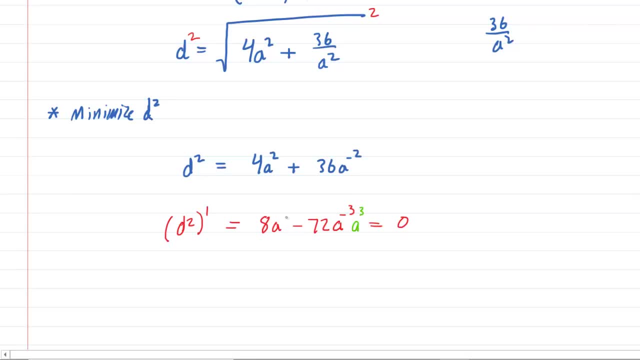 every term by a to the positive 3, just like this. And what's nice about that is you end up with, let's see, 8a times a cubed. That's going to be 8a to the fourth. These, when you multiply them, become a to the zero. Remember you have to add 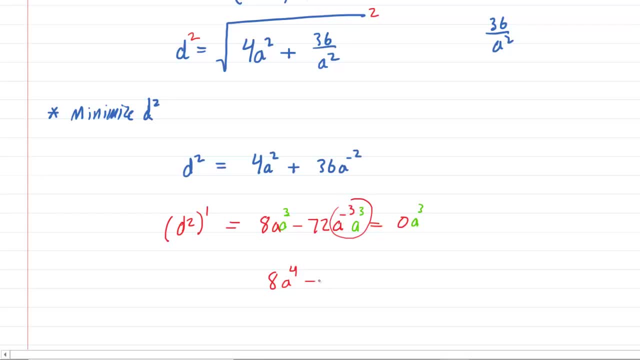 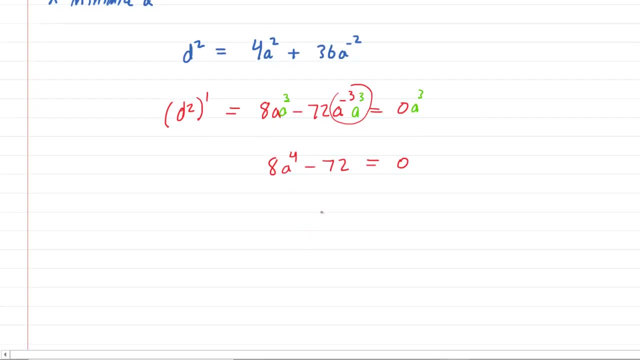 the powers, But a to the zero is just 1.. So this is 8a to the fourth, minus 72 equals the other side is still 0. And now it becomes a lot easier. There's no negative exponent, So add the 72 over. 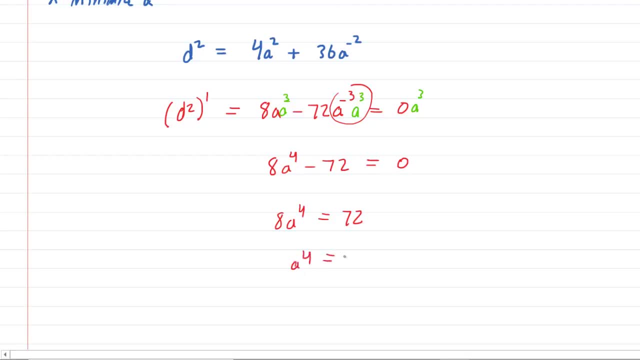 divide both sides by 8, and you get a negative exponent. So that's going to be a negative exponent. So that's going to be a. And then take the fourth root, So we can see that a is going to equal the fourth root of 9.. 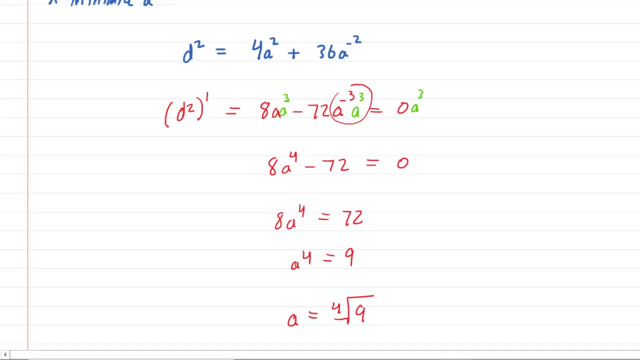 Not a very pretty number, but certainly a correct number, And your teachers might require you to prove that this actually minimizes the d squared function. So to actually prove that it minimizes the d squared function, you could actually do the second derivative test. 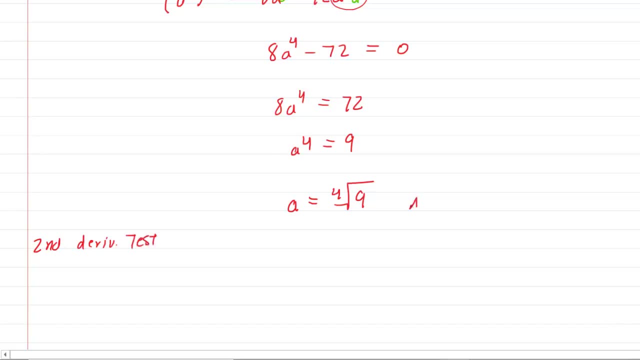 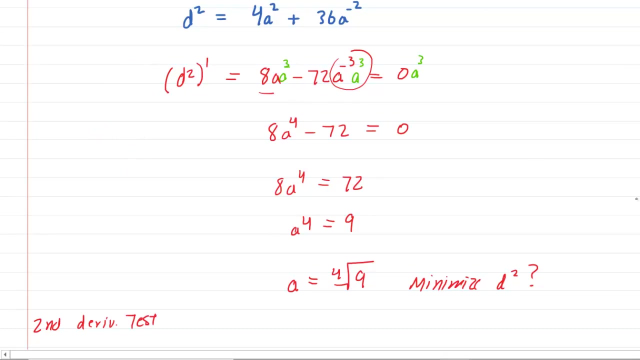 Some teachers kind of omit this. but just to make sure that this indeed minimizes the d squared, we're going to do the second derivative test So we can go back and snag our first derivative, which was: yeah, right. here It was the 8a minus 72a to the negative 3.. 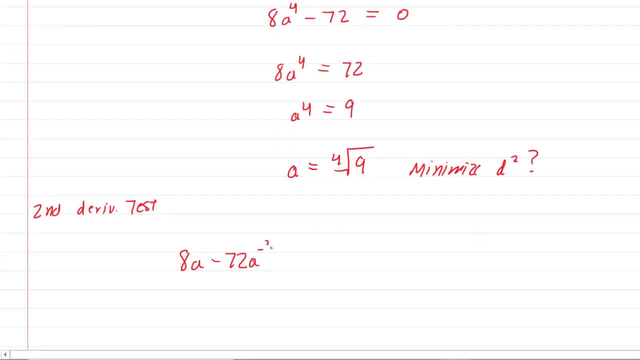 8a minus 72a to the negative 3.. That was our first derivative. Let's do the second derivative now. So this would give us 8 plus whatever. 72 times 3 is 216. And then a? a to the negative four. that can be rewritten. 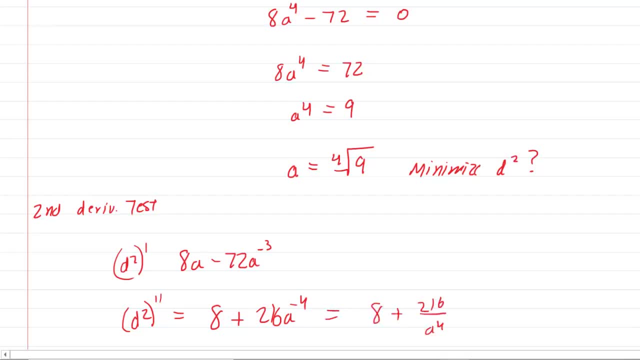 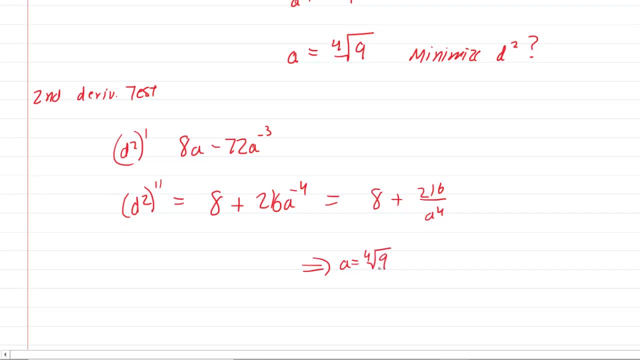 as eight plus two, 16 over a to the positive four. Now, certainly if we plug in our a here- if we plug in our a is equal to the fourth root of nine- we're gonna have eight plus two, 16 over the fourth root of nine to the fourth. 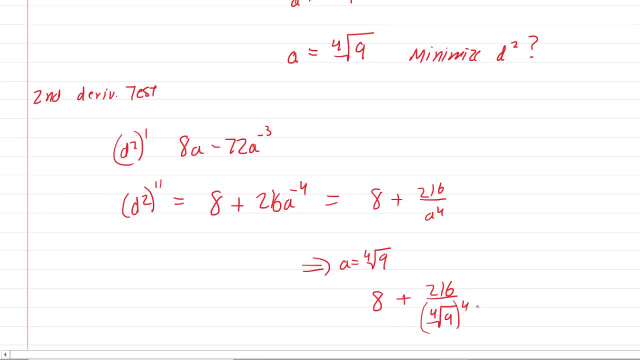 And that, indeed, it actually doesn't even matter what the value is, but all you need to note is that that is greater than zero, And so when the second derivative is greater than zero, in other words it's positive. you might remember that that means the function. 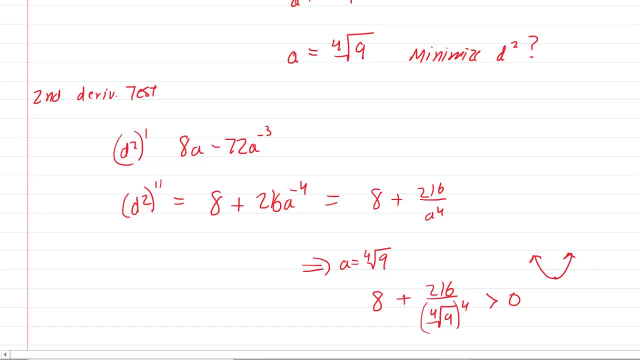 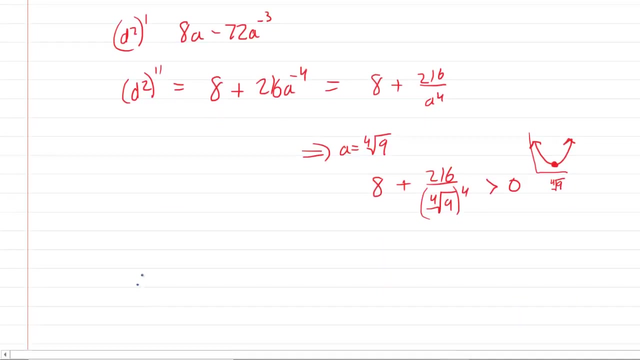 is concave up. Well, a concave up function located at this little critical point of fourth root of nine would indeed be a minimum. So we've proved that at the fourth root of nine we minimize the d squared function. So, in conclusion, we now know that a is equal. 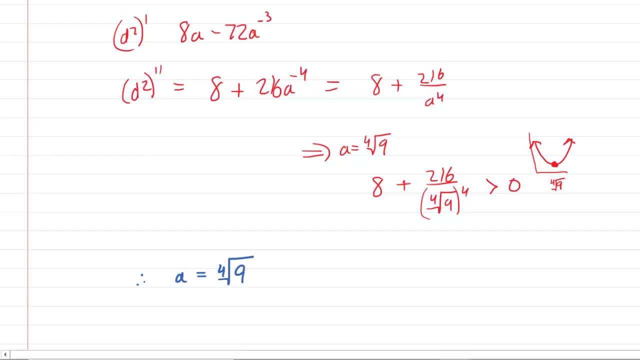 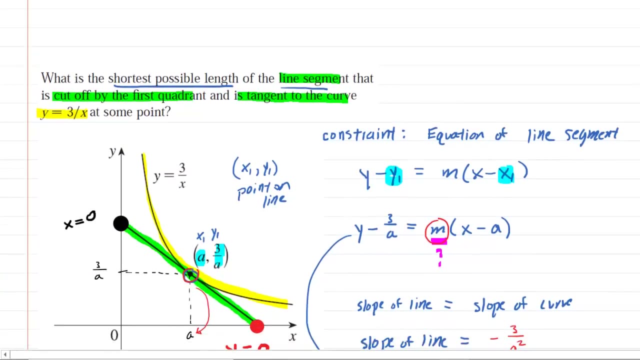 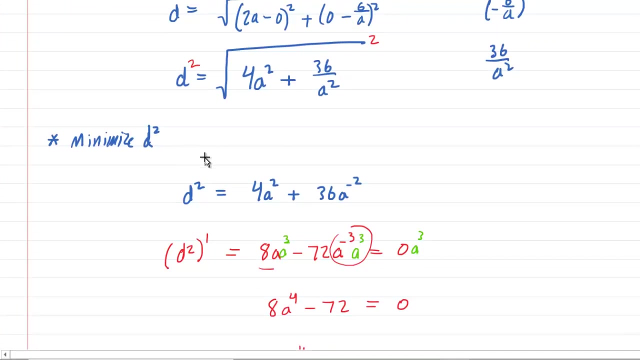 to the fourth root of nine. Let's make sure we're not forgetting. we've actually answered the question. The question is to actually find the length. So we haven't yet answered the question. We have to find the actual length, And so let's see here. here is our d squared function. 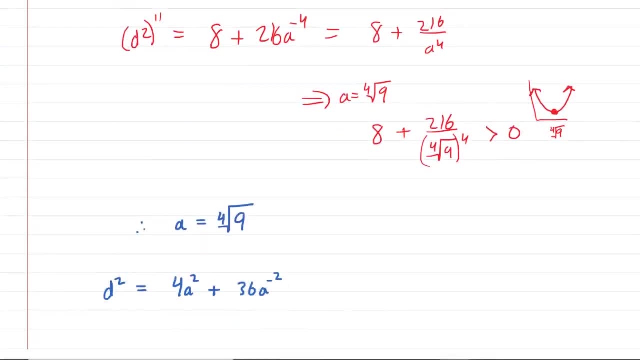 What we're gonna need to do is still find d. That's what the question is asking us is to find d. So that's what we're gonna do right now, And we might find it useful before we plug in the fourth root of nine. 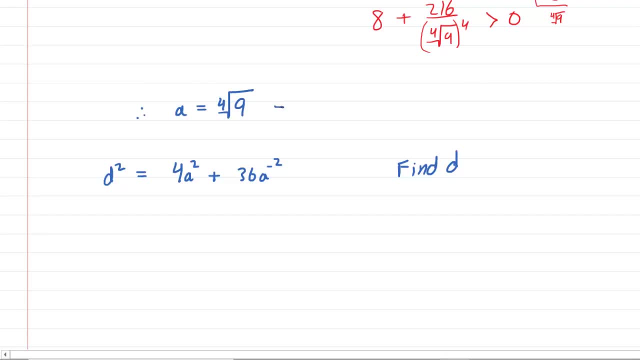 is to maybe rewrite that. And so let's see the fourth root of nine that can be rewritten as nine to the power of 1. 4th, We can rewrite nine as three squared. But then when you multiply these exponents, 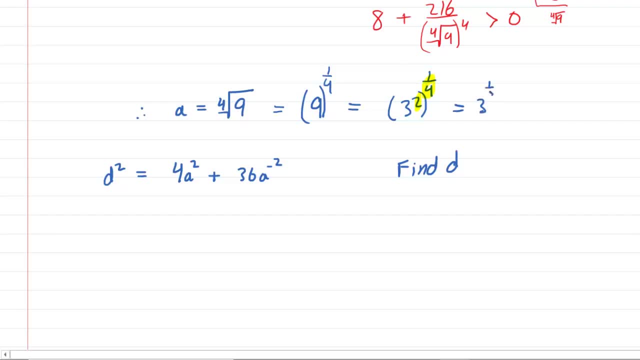 you would end up with three to the 1: 1⁄2, which is the square root of three. So that's just a little way of rewriting the fourth root of nine. It's actually equal to the square root of three. How about that?